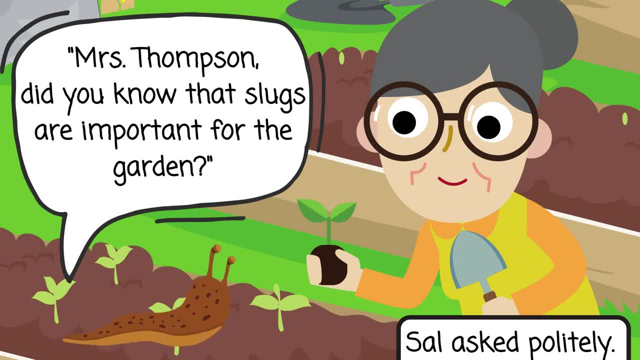 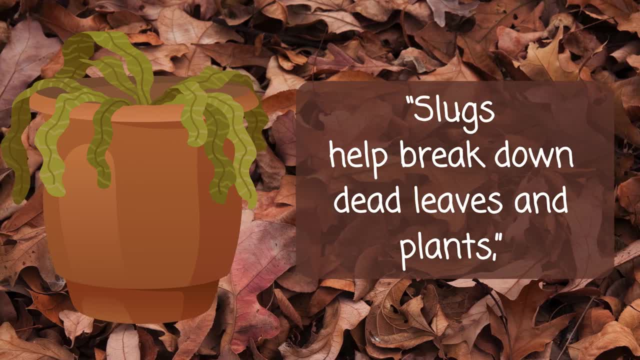 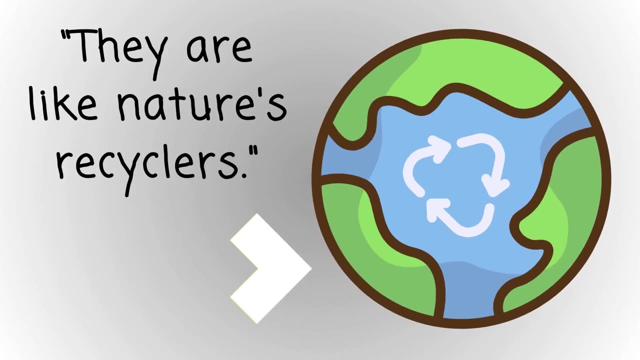 are important for the garden? Sal asked politely. Mrs Thompson smiled. Of course Sal. Slugs help break down dead leaves and plants, turning them into nutrients for the soil. They are like nature's recyclers. Sal nodded: That is right, but some people use salt on slugs. 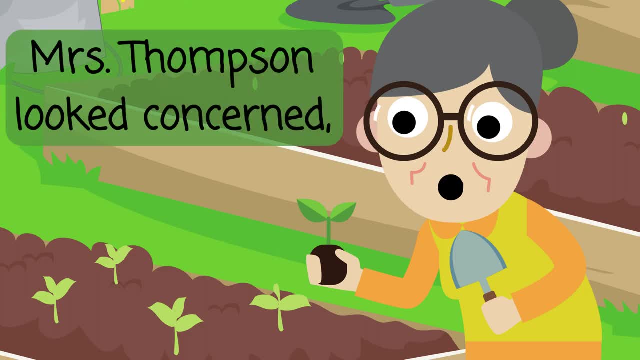 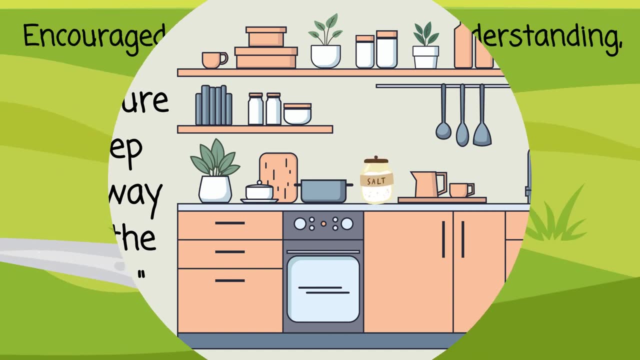 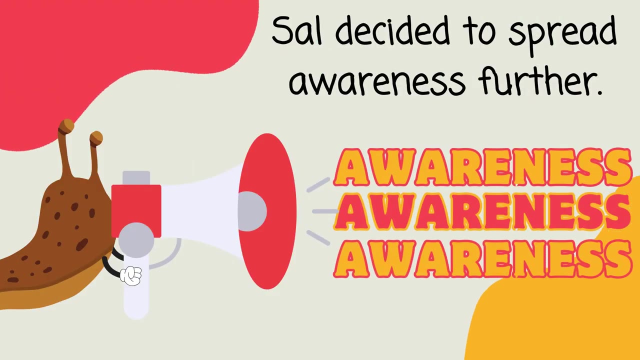 Which can harm us. Mrs Thompson looked concerned. Oh dear, I did not know that. I will make sure to keep salt away from the garden. Sal was encouraged by Mrs Thompson, He said Sal decided to spread awareness further. He organized a slug safety day in the garden. 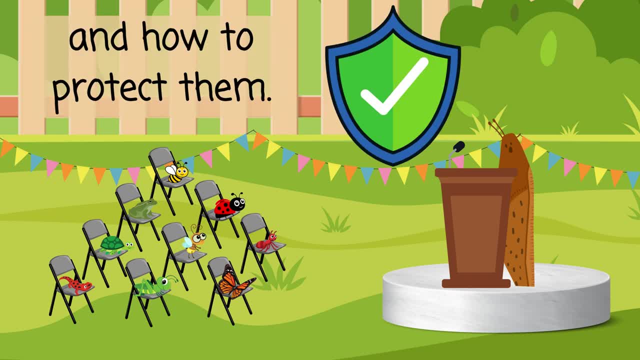 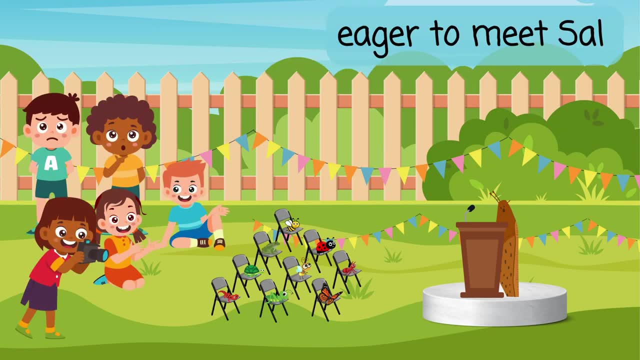 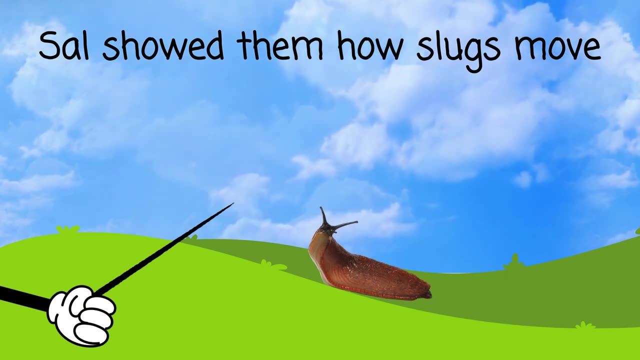 inviting all the creatures to learn about slugs and how to protect them. Other children from the nearby school joined in, eager to meet Sal and learn about his slimy adventures. Sal showed them how slugs move and how they leave a trail of slugs. 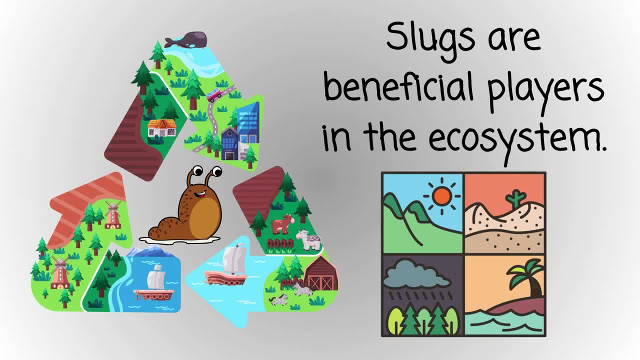 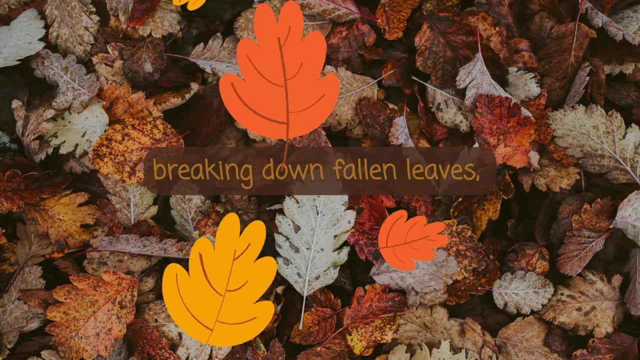 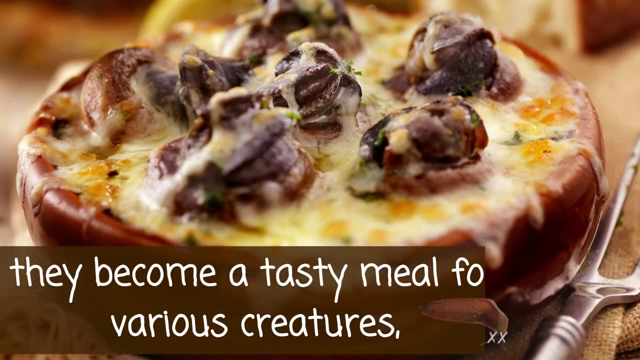 Sal told his children that it is a good idea to stick a slug in your yard. Slugs are good players in the ecosystem. Many slug species function as nature's recyclers, breaking down fallen leaves, deceased insects and even worms. On the flip side, they become a tasty meal for various creatures, including snakes, toads. 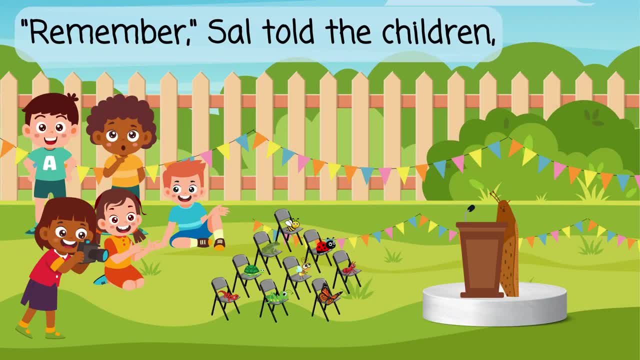 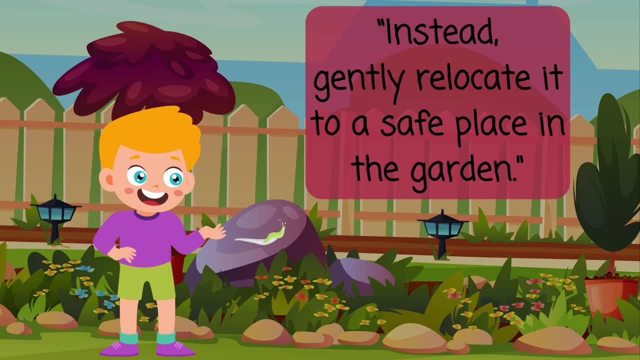 burtels and birds. Remember Sal told the children: if you ever see a slug that is ornaments- every slug moves and becomes important to this garden- do not use salt on it. instead, gently relocate it to a safe place in the garden. the children 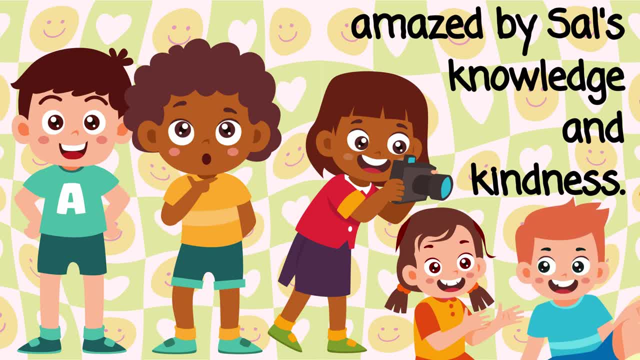 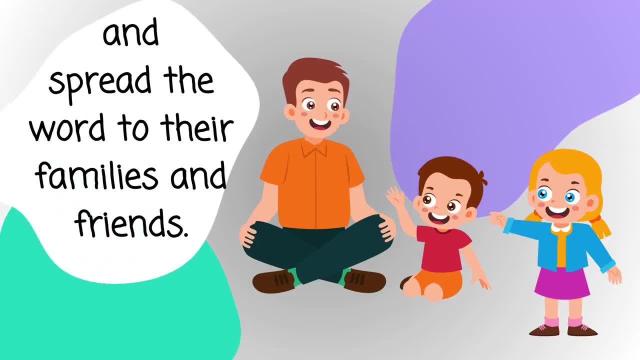 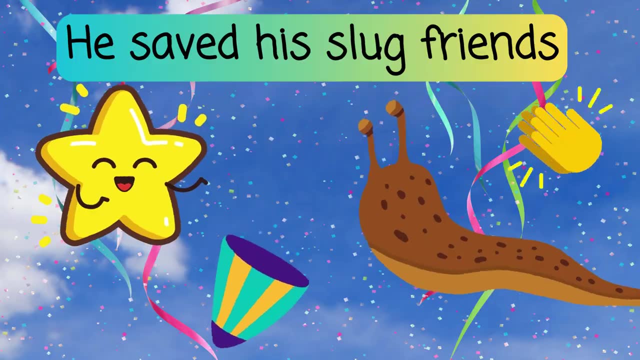 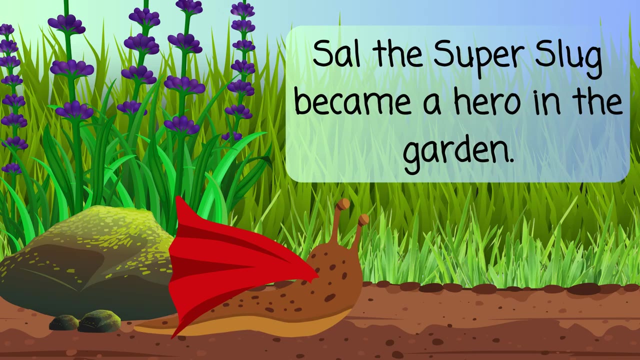 nodded. amazed by Sal's knowledge and kindness, they promised to be slug protectors and spread the word to their families and friends. as the day ended, Sal felt happy and proud. he saved his slug friends and taught others about the value of all creatures, big and small. from then on, Sal the super